that is aging and research is going to use thymus. So 25% of people are going to use thymus. We can say that 50% of the population that is aging and research is going to use thymus, So that's a significant improvement for our population. Dr Dan Weissman- So actually the significant effect of these changes is not very significant. I mean, we can talk about paniomycin. I think that there are a number of reasons that we can talk about, but one is there's. a better progression of thymus. I can tell you one of them is: there's a good reason that thymus is a good institution, and that is that we are at the end of the world. we can think about what we are at, but it's not a perfect issue, because it's not just 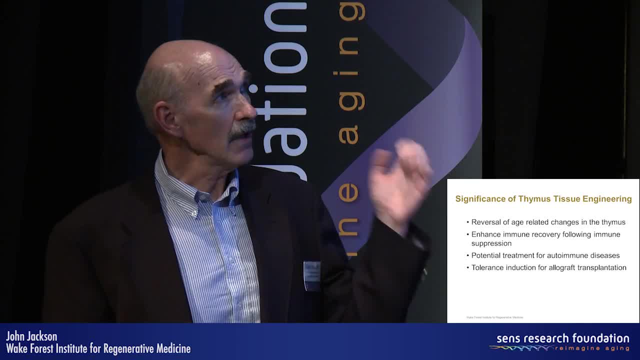 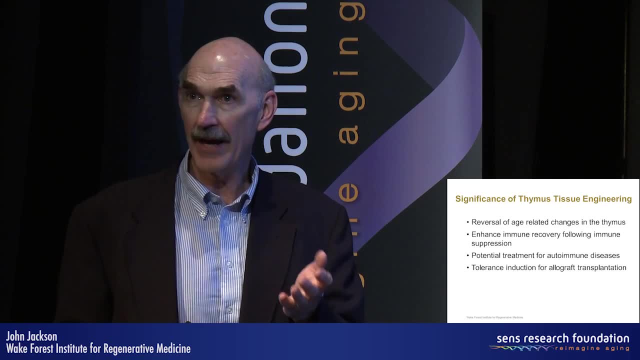 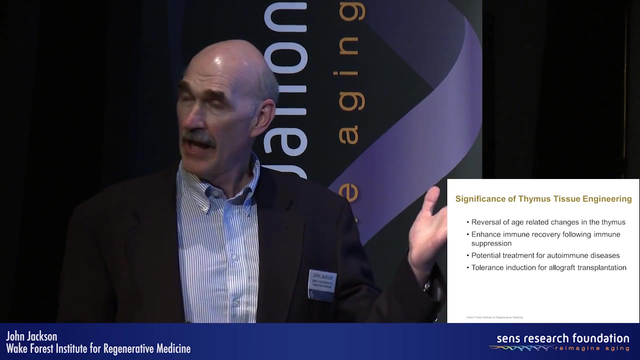 an issue, particularly in cancer treatments, potential treatments for autoimmune disease. You may be able to reset the immune response in people that have autoreactive T cells. And also tolerance induction in allograft transplantation. You may be able to induce central tolerance. 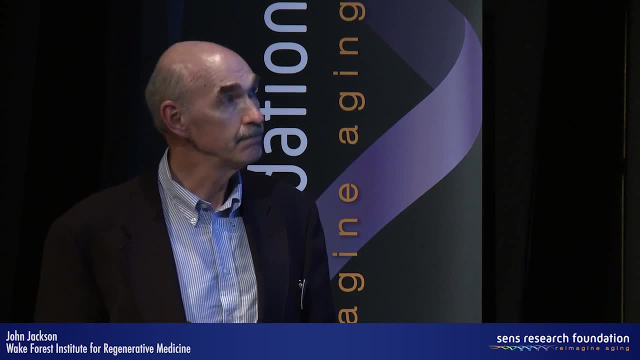 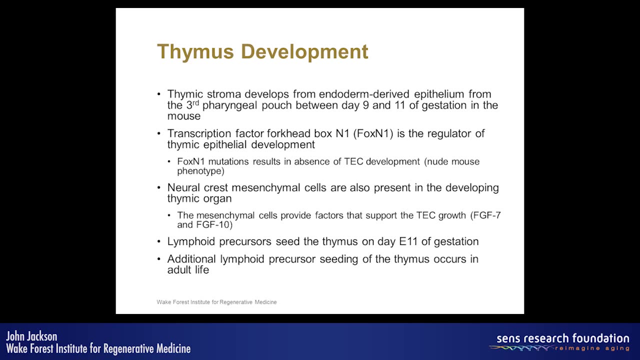 and get rid of immunosuppression in these transplant patients. So just a little background on the thymus. It develops from endoderm that's derived from the third pharyngeal pouch during embryological development. One of the important transcriptional factors is FOXN1. 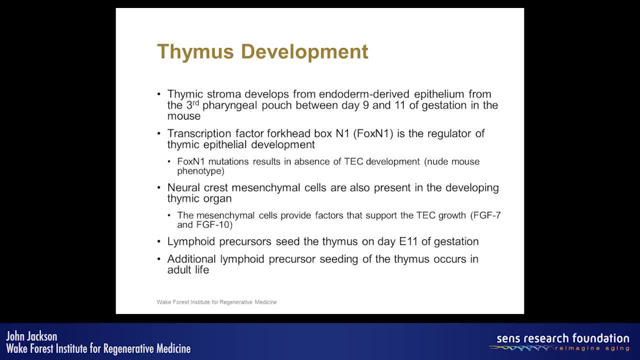 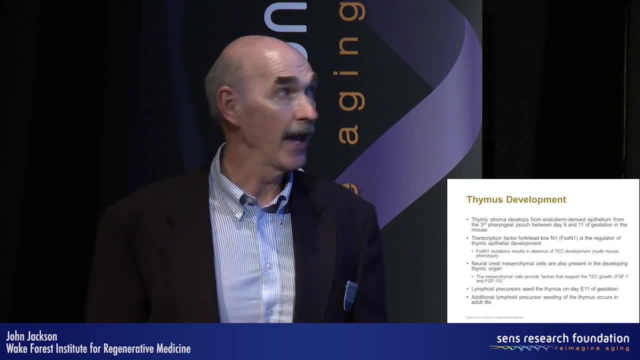 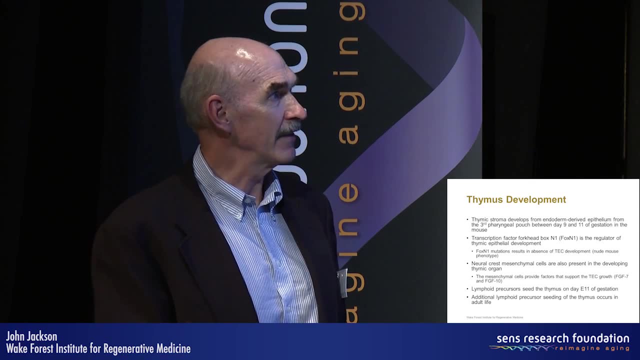 Without that you get no thymic epithelial seeding of the organ And the phenotype is the nude mouse. It's an athymic animal. You also get some neural crest mesenchyme cells present with the thymus. It's in the developing thymic organ. 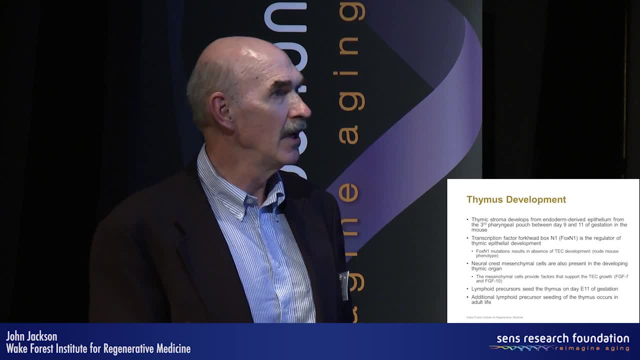 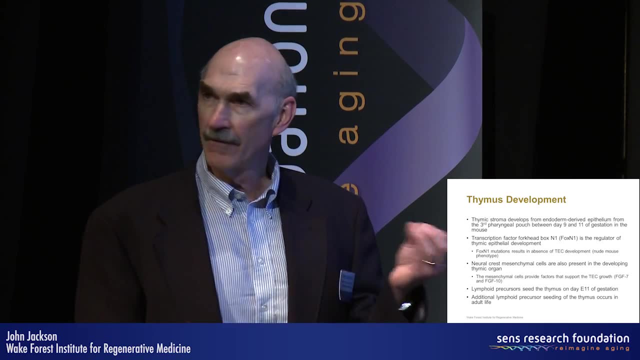 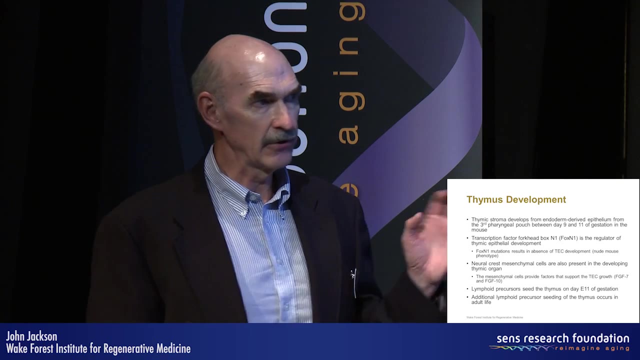 These provide some of the support growth factors for thymic epithelial cells, Lymphoid progenitors from the bone marrow seed, the thymus, very early in embryological development And there is evidence that you also get additional lymphoid precursor seeding. that occurs in waves during adult life. 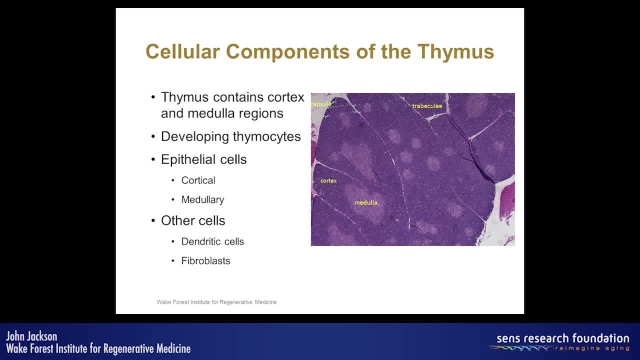 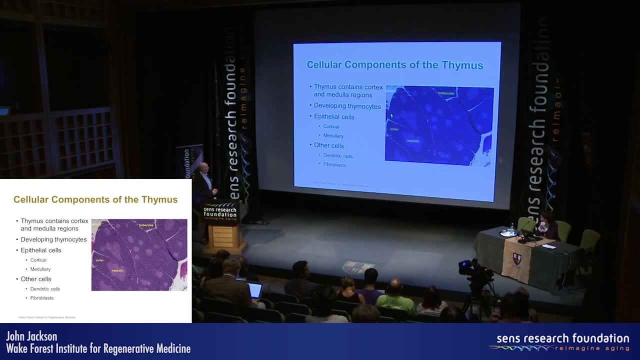 So this is a picture of the thymus It contains. There's a cortical region and a medullary region, And there are specific cell populations of epithelial cells in these two regions. There are cortical epithelial cells and medullary epithelial cells. 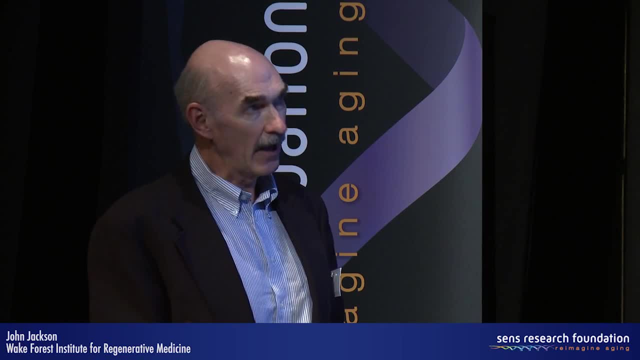 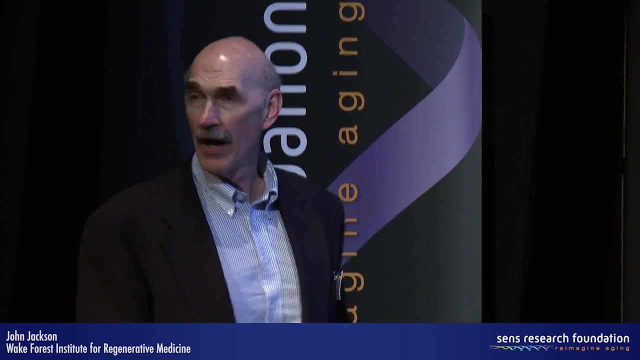 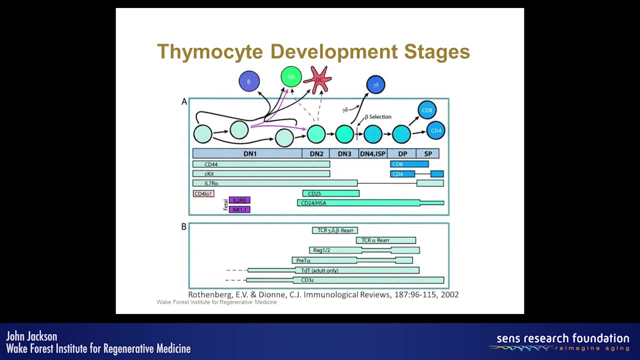 And they have different functions. Other cells that are very important in terms of education of the T cells in the thymus are dendritic cells And I said some of the fibroblasts provide some of the growth factors. This is a schematic diagram of some. 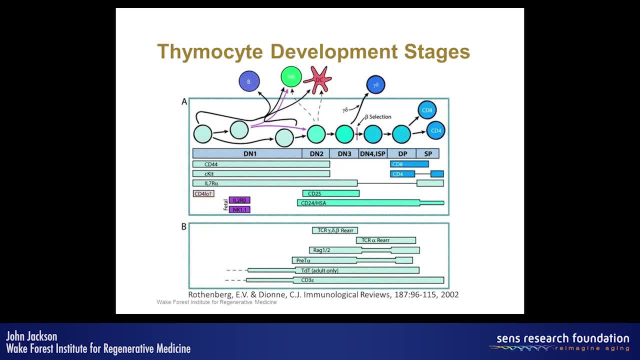 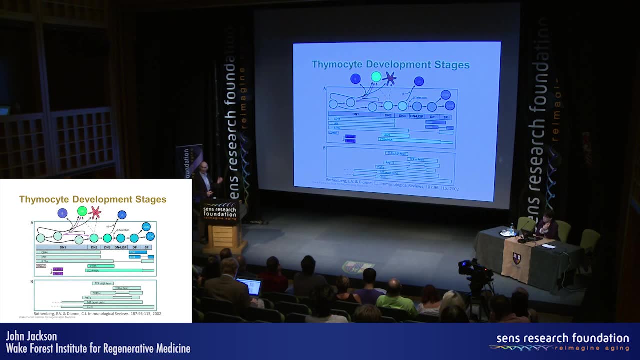 of the early developmental stages of thymocytes as they develop, mature in the thymus, And it's been fairly well characterized And there are different stages here, denoted by DN1,, 2,, 3, 4. This stands for double negative. 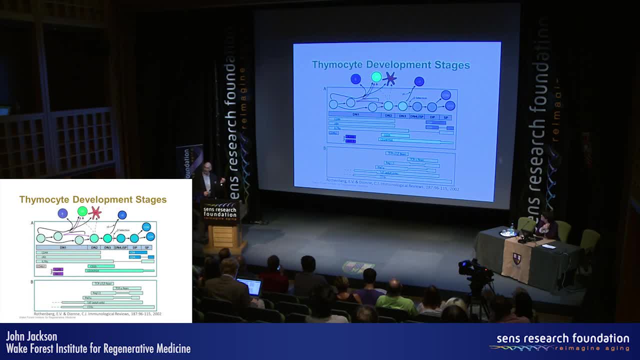 And if you look at these thymocytes, you have CD4, CD8, and they don't express those, And that's why it's termed double negative, And then you come into a double positive, So it expresses both CD4, CD8.. 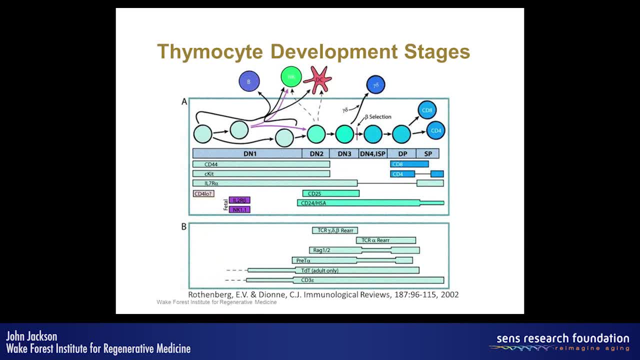 And then final maturation of a single positive. It chooses between the CD4 expression or CD8.. CD4 gives you hepar T cells, CD8 positive cells or cytotoxic T cells And you can look at other. So it's a combination of CD4 and CD8. 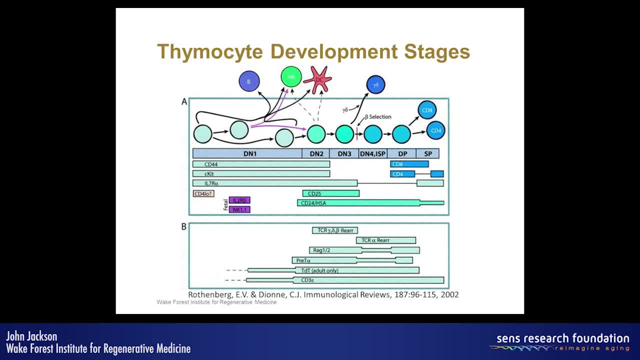 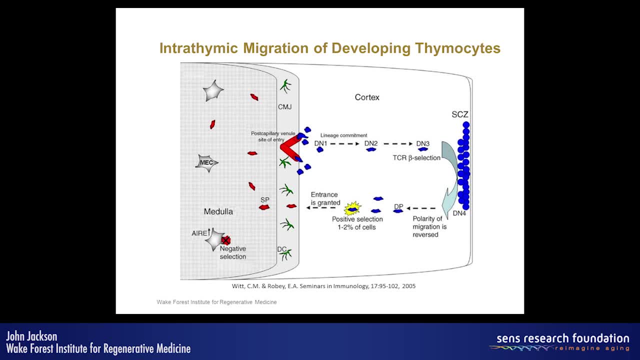 Surface markers, expression of certain cytokines, are very important during this developmental stage, as well as gene rearrangements for the T cell receptor. There's a very specific and unique pathway for these developing thymocytes: They come in from the bone marrow. 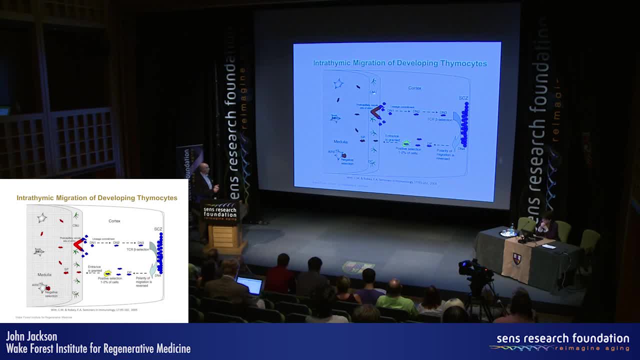 bone marrow precursor cells come into the corticomedullary junction area, They start their maturation process and they start a migratory pathway from the corticomedullary junction toward the capsulary region within the cortex. They undergo their maturation process. 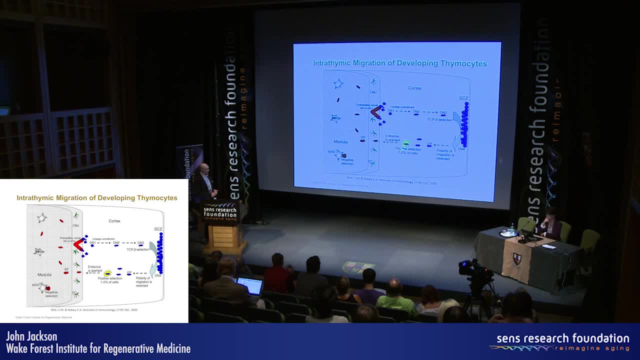 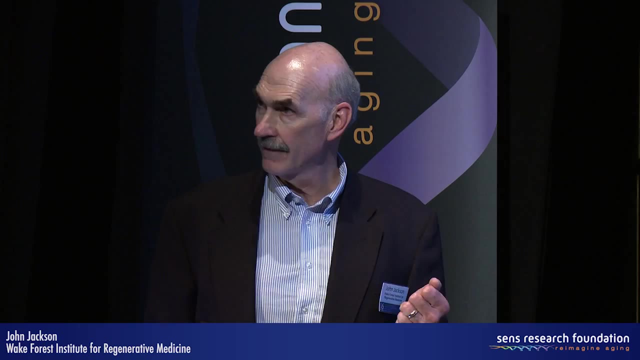 During this part a very important selection process. a positive selection occurs. They then mature to single positives, move into the medulla medullary region and then they undergo negative selection, hopefully to eliminate any self-reactive T cells, and then they exit the thymus as mature cells. 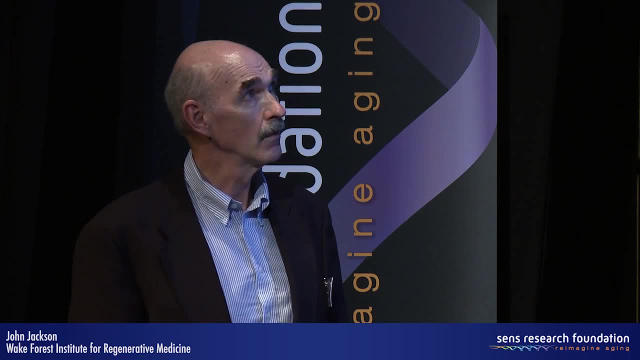 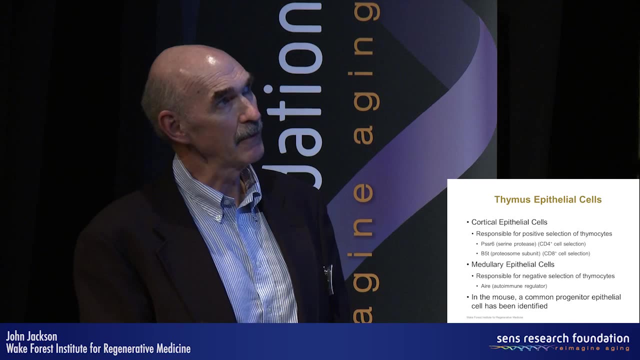 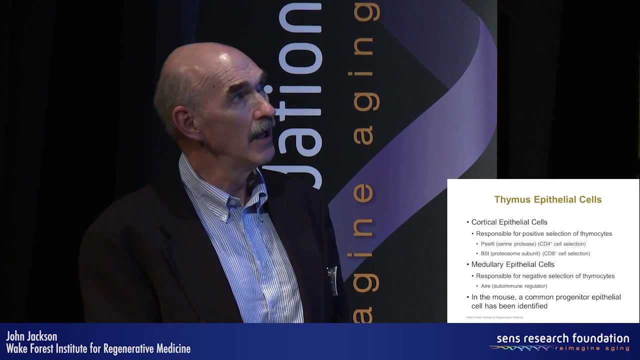 to go to the periphery Now. as I said, within the thymus there's cortical epithelial cells. Those are responsible for positive selection of thymocytes. There have been a couple of molecules here: the serine protease and a proteasome subunit. 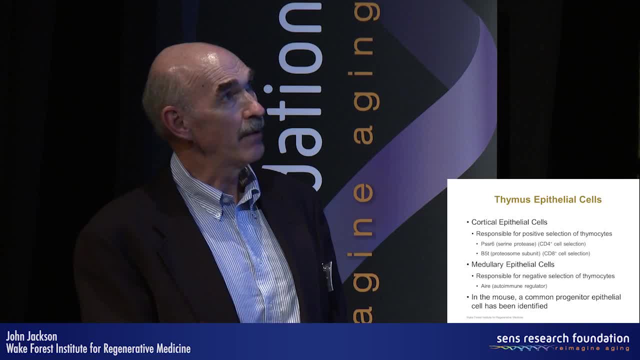 that have activity in this positive selection. This positive selection of specific CD4 and CD8 populations And the medullary epithelial cells help in the negative selection. of thymocytes as well as some dendritic cells are very important in the negative selection. 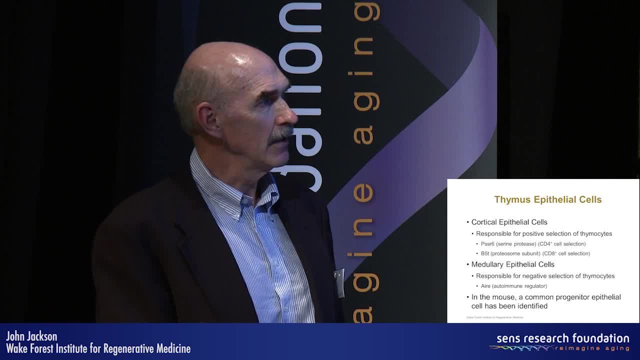 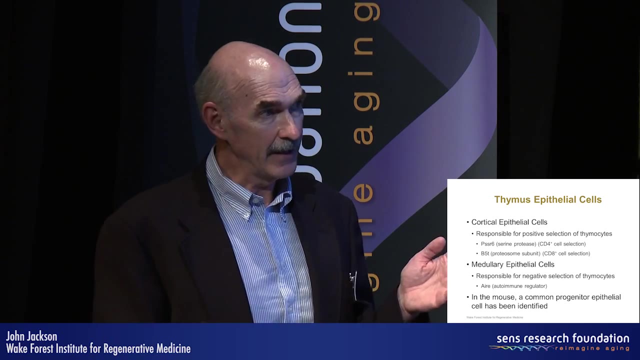 And all this is associated with an autoimmune regulator transcriptional factor called AIR, And in the mouse a common progenitor epithelial cell has been identified, particularly in the embryological developmental stage. There's been some difficulty identifying this in the adult animal. 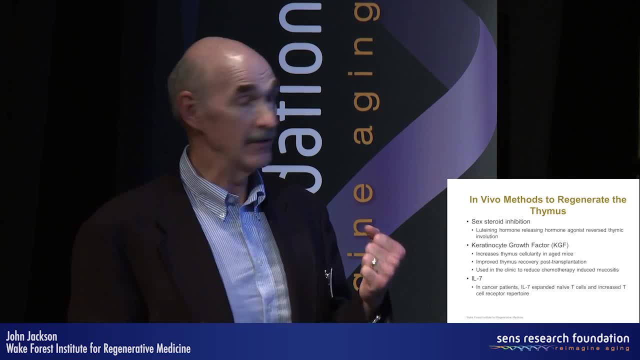 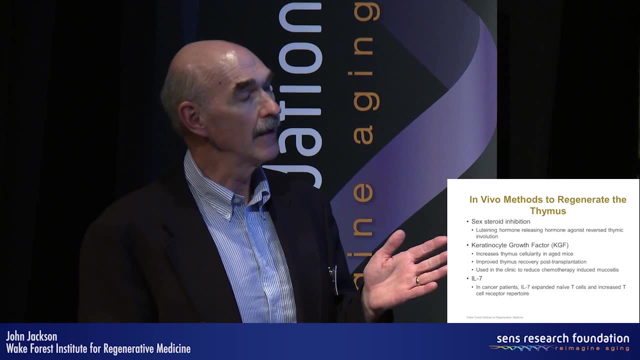 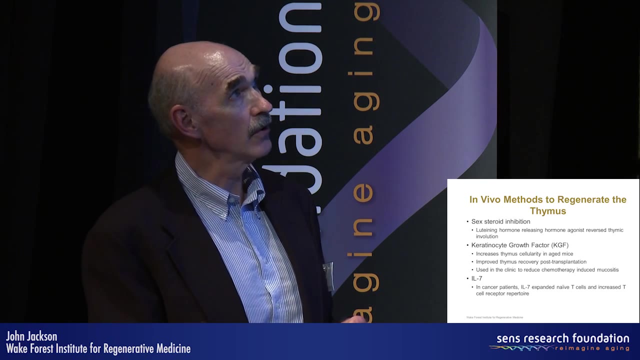 As we age the thymus involutes or decreases in size. There have been attempts on the clinical side to reverse some of that degradation of the thymus And one of those is you can inhibit some of the sex steroids by using the luteinide hormone releasing hormone. 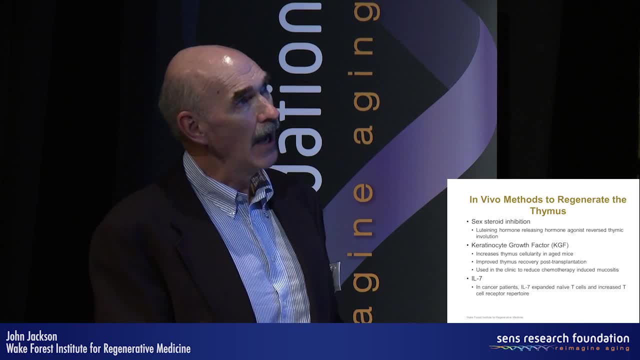 agonist and that reverses some of the thymic involution. Growth factors, such as keratinocyte growth factor, has been used. It increases some of the cellularity within these aged mice And clinically it has been used in chemotherapeutic patients. 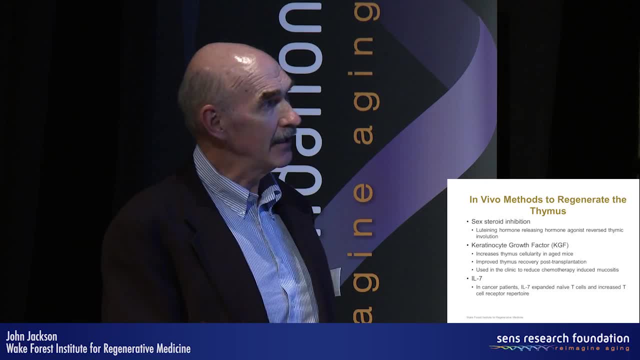 to reduce some of the mucositis. A cytokine that's very important is interleukin-7.. In some cancer patients IL-7 expands the naive T-cells and increases the overall T-cell repertoire. But again, this is These are all transient. Once you stop treating, the effects go away within the thymus. There have been a number of ex vivo T-cell production assays, developed many years ago in terms of using both thymic stromal layers that contain the epithelial cells. 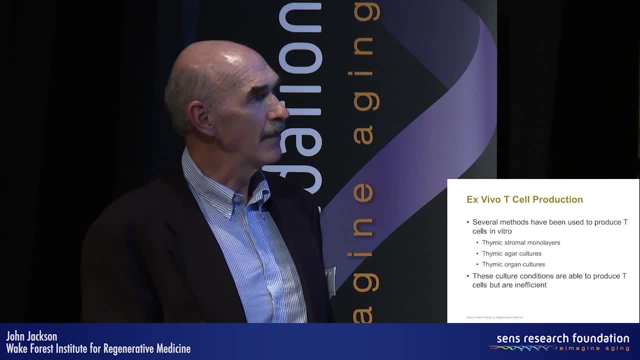 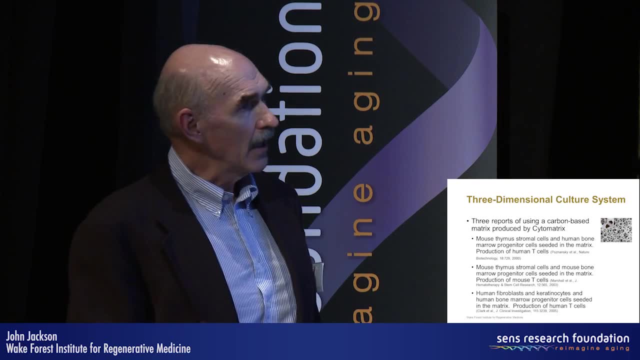 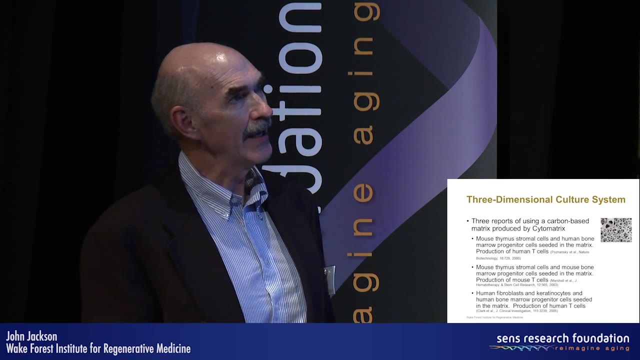 some agaric cultures and thymic organ cultures. These do produce T-cells, but the whole process is very inefficient. There was a group of about three publications that occurred in the early to mid-2000s using a solid matrix material. 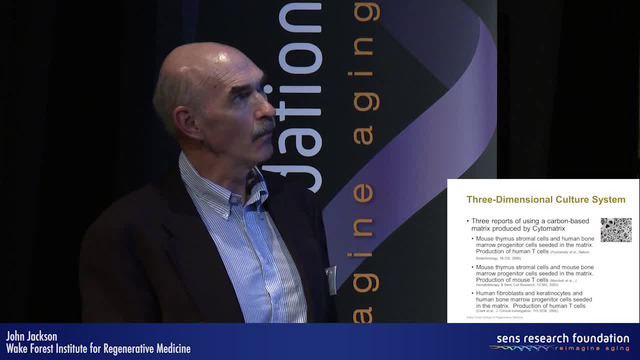 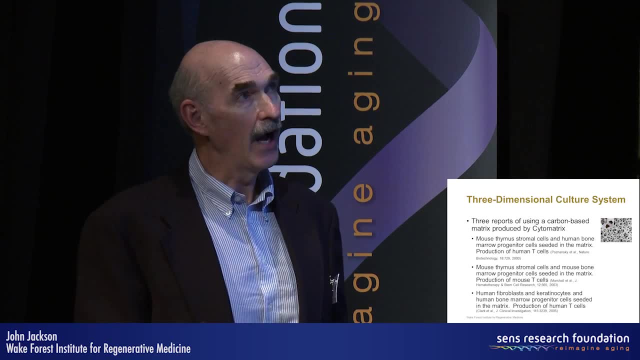 It's a carbon-based matrix And they seeded them with thymic stromal cells and bone marrow progenitor cells and they could get T-cell production out of this 3D or three-dimensional culture system. And, very interesting, there was one publication that used human. 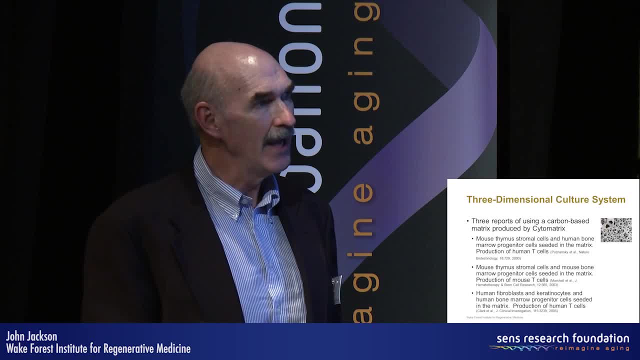 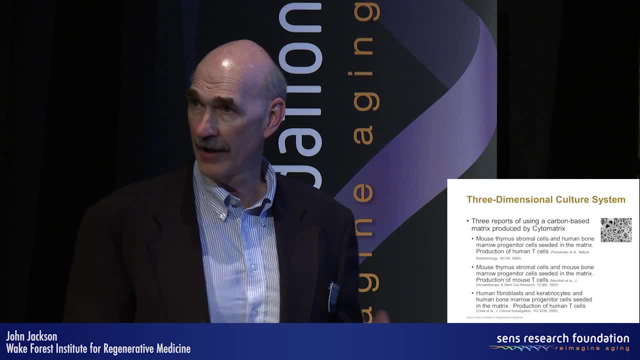 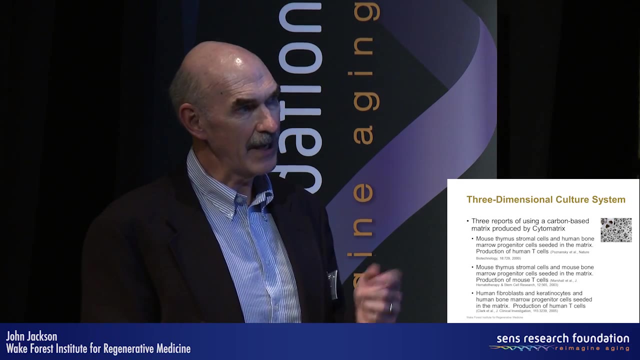 fibroblasts as well as skin keratinocytes from humans, and they found that this was able to produce T-cell maturation. But there's some controversy in terms of using keratinocytes. They express some of the similar markers as thymic epithelial cells. 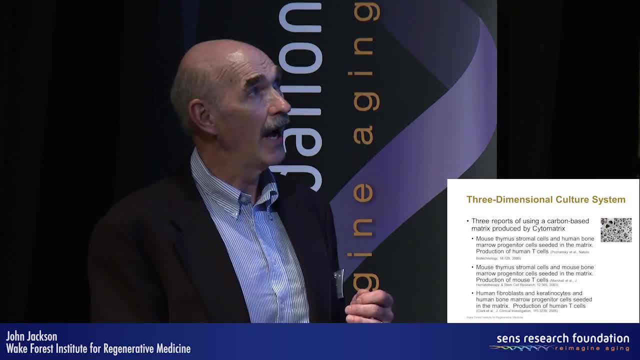 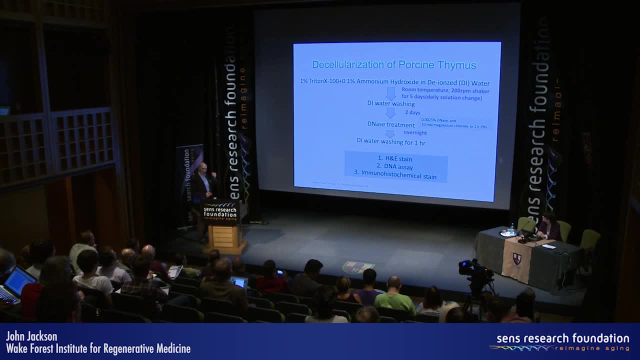 but this is an ectodermally derived epithelial cell. Thymic epithelial cells are endodermally derived, So we wanted to. We wanted to approach this in terms of using a scaffold, But we chose to use a natural scaffold through a decellularization process. 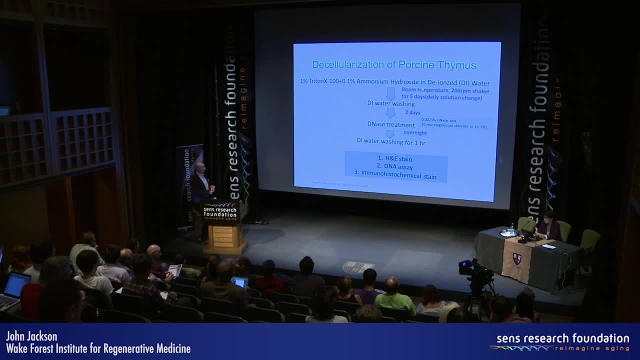 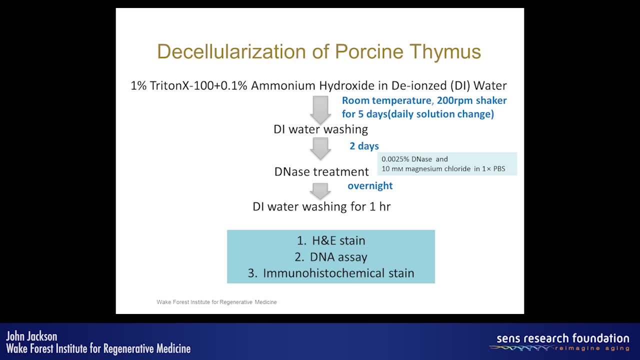 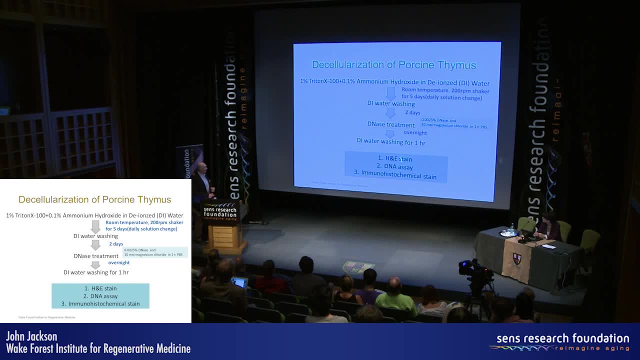 I'll show you a little bit of data that that may or may not be the best way to do it. I'll show you a little bit of data that that may or may not be the best way to do it. And then more washing, and then we're looking at different assays to characterize these scaffolds. 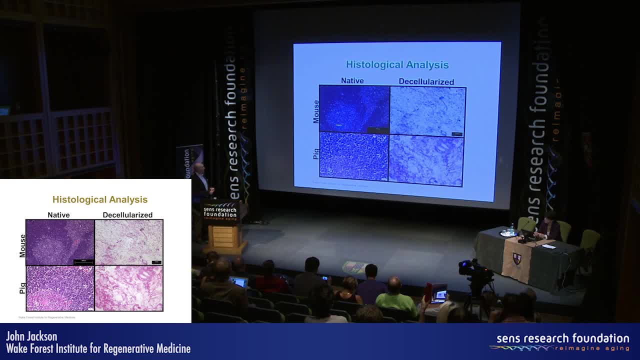 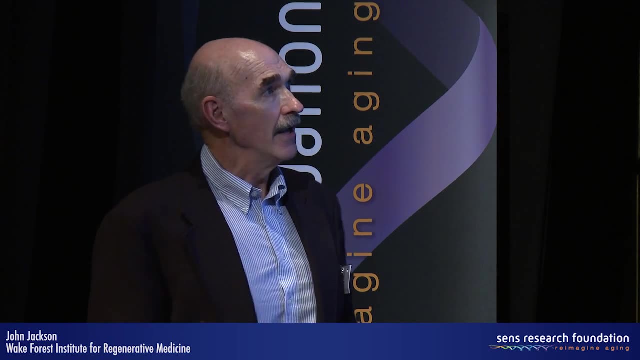 So this shows an HE-stain of a native thymus tissue, both mouse and pig medullary region, cortical region. This is after decellularization and you've got the matrix material. that's the only thing left If you look at the DNA after a decellularization. 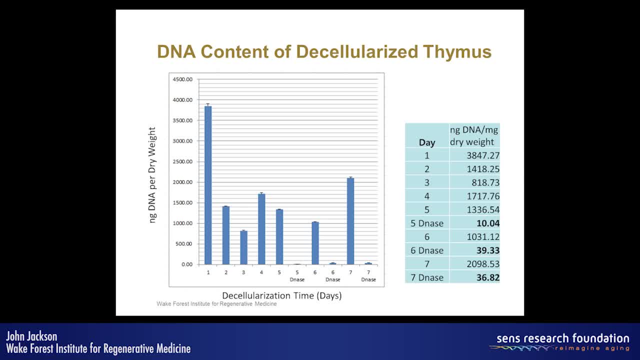 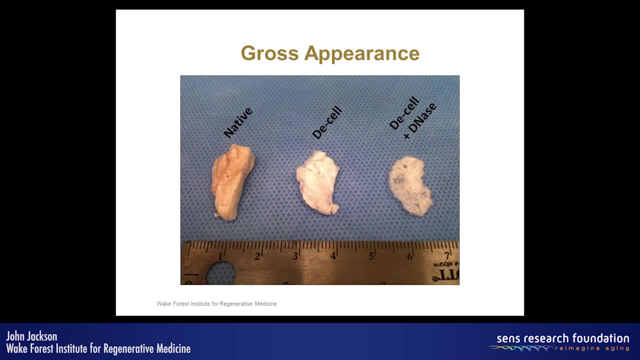 After two days of decelerization you can see significant reductions in the amount of DNA. but if you use DNAs, you can almost eliminate any of the DNA present on that scaffold material. However, if you look at this, this is native tissue. this is freeze dried material. this 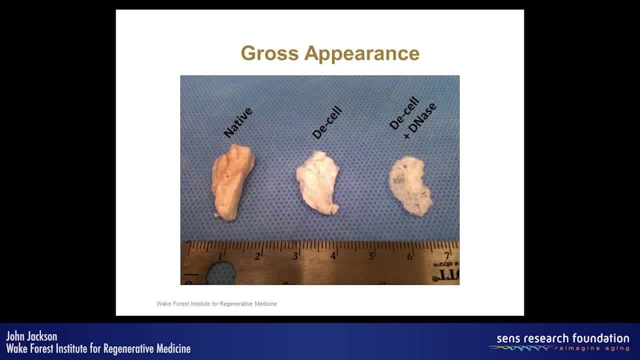 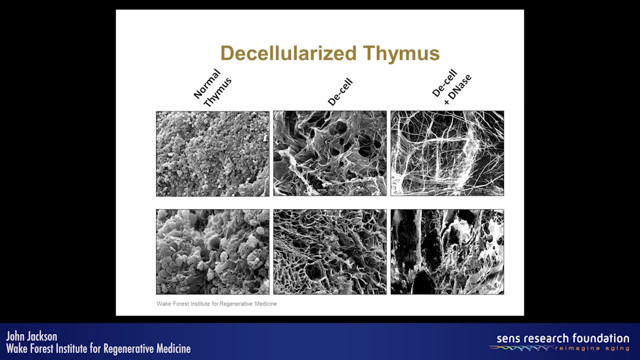 is after decelerization and then if you look after DNAs treatment, you can see significant degradation of that scaffold. So we're concerned in terms of what's happening during this process. This also can be seen in scanning EMs. This is the decelerization picture of the decelerization of the scaffold and then after. 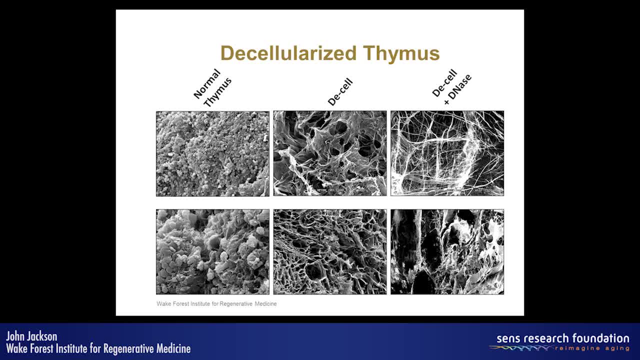 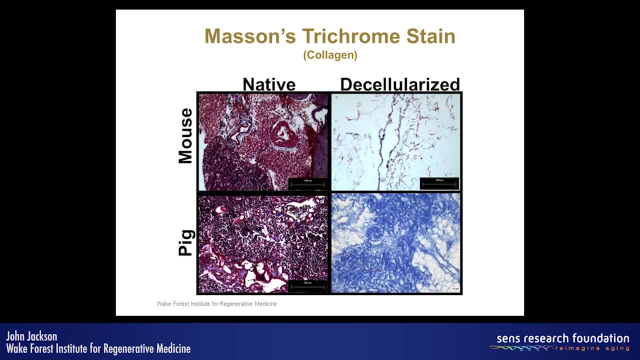 DNAs treatment And you can see, appears to be significant damage to the scaffold after this treatment. We want to talk about the DNA analysis. We want to talk about the DNA analysis. We want to talk about the DNA analysis to characterize what molecules were present on the scaffold. 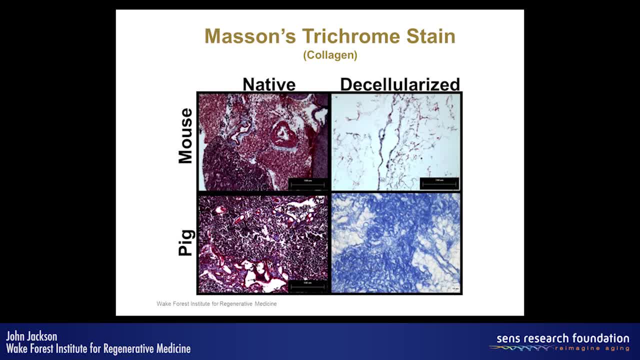 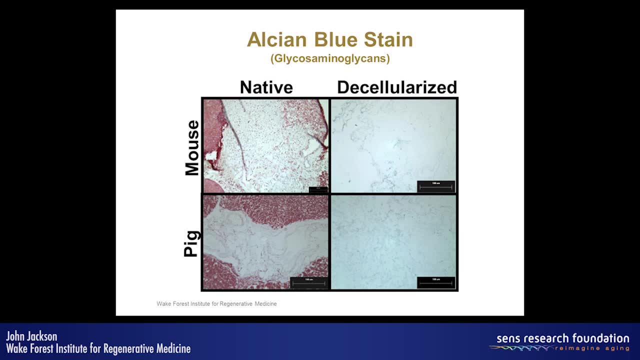 This is native tissue stained with a Mason's trichrome which stains collagen blue. in the mouse You can see there's still a little blue remaining in the scaffold. In the pig there's much more dense collagen remaining in the scaffold And, using Alcyon, blue stain looking. 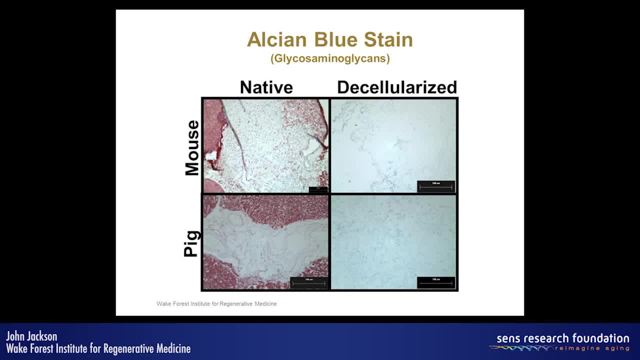 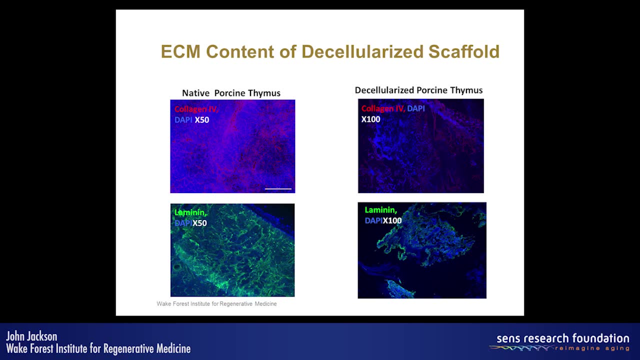 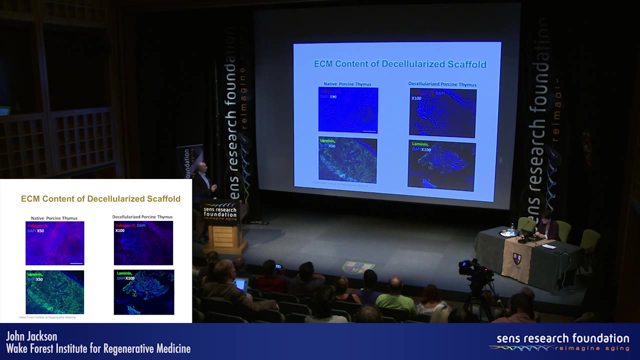 at glycosaminoglycans. very little is remaining in the scaffold, So we have some problem in terms of this whole procedure eliminating some of the ECM components. Now we also further characterized these scaffolds looking at collagen, specifically collagen 4.. 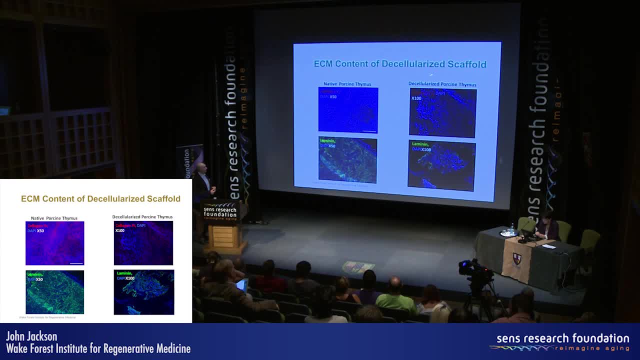 This is a native thymus tissue And this is after decelerization And you can still see some of the collagen. 4. present laminin in the native tissue and you still see some present in the decelularization. 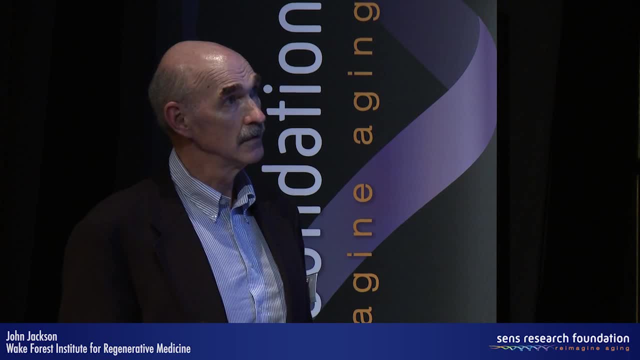 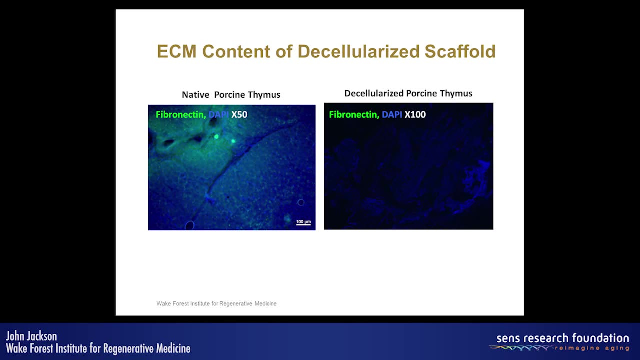 following decelerization of the scaffold. Now, with fibronectin, it's a little bit different story. We have significant amounts of fibronectin in the native thymus, but it's almost completely eliminated during the decelerization process. 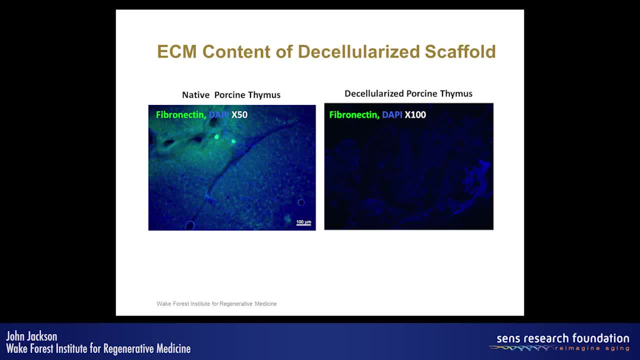 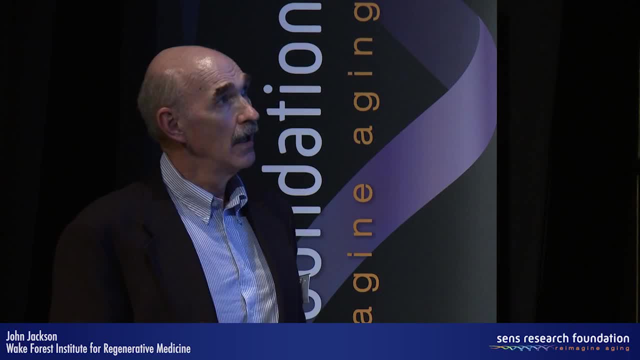 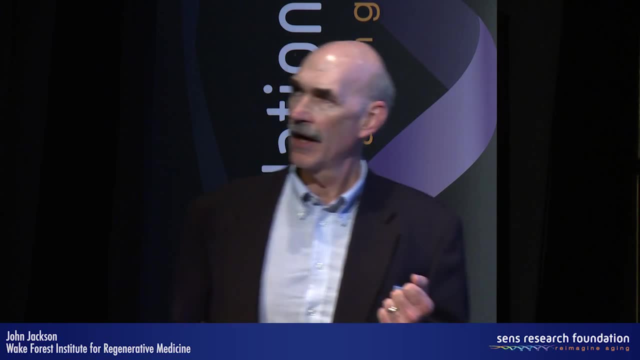 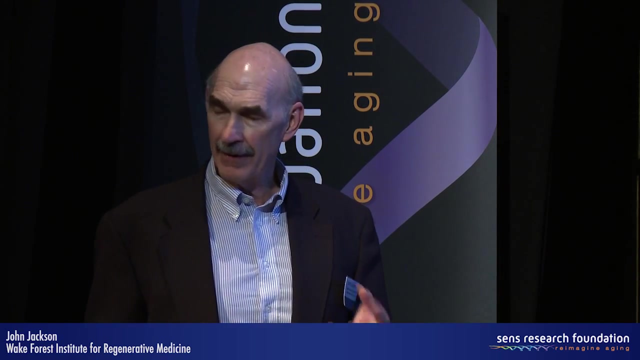 So this is one of the molecules, And it appears to get washed away or eliminated during this whole process. So one of the things we wanted to look at, then, is how effective will these scaffolds be in terms of enhancing proliferation of epithelial cell? 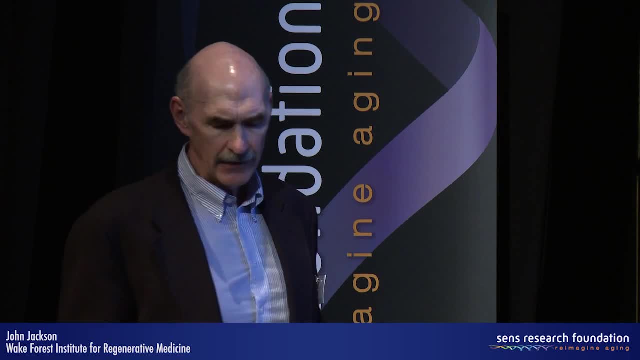 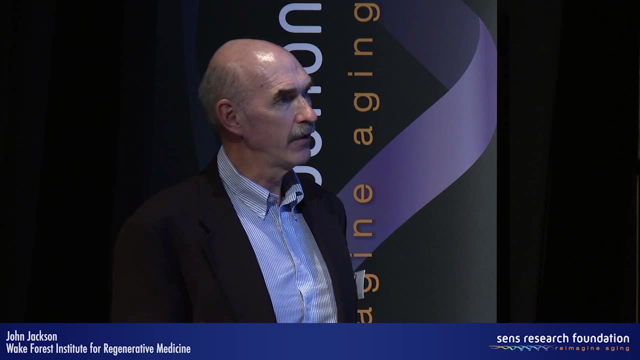 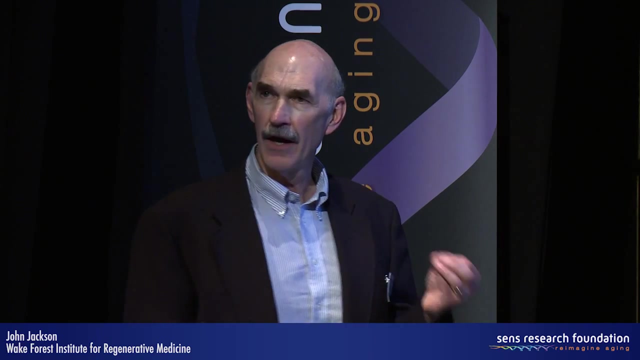 populations, maintaining their phenotype and culture. So what we did was we looked at The decel thymus scaffold from a porcine model, as well as taking whole thymus tissue that we freeze, dried and cryo-milled and made a powder. 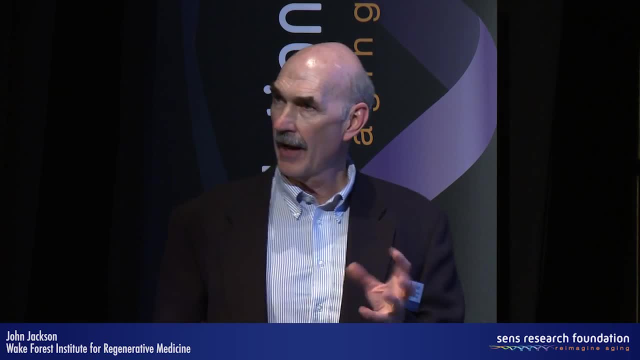 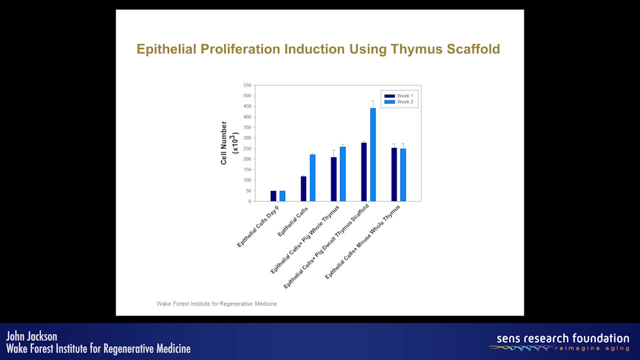 And we did the same thing with the scaffold. We cryo-milled it and made it a powder, And we also looked at the mouse hole thymus as a cryo-milled powder, And if you add that to two-dimensional cultures of epithelial cells, 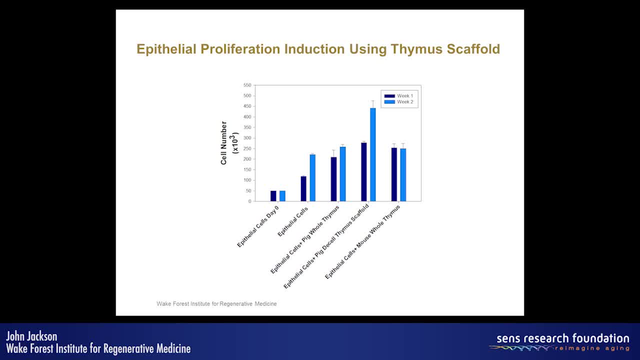 And you plate the epithelial cells. After one week the epithelial cells do undergo proliferation, But in the presence of the scaffold or cryo-milled material from the thymus we see an enhanced proliferative response And after two weeks the decel thymus scaffold 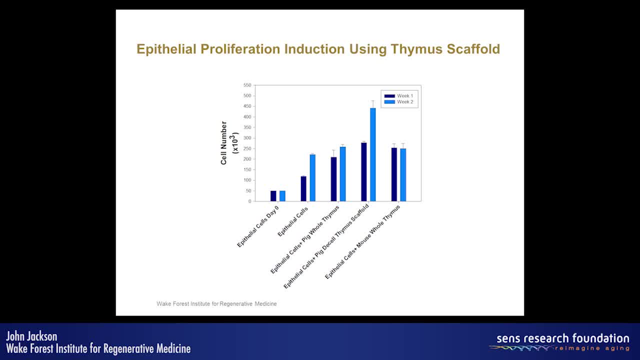 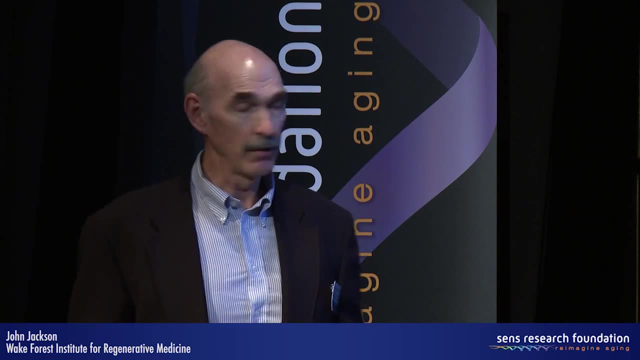 actually gave us the best results And we're not sure why we didn't continually see proliferation after two weeks with the whole thymus from pig or from mouse. It may also contain some inhibitory activity for proliferation. We have to actually look at this a little bit closer. 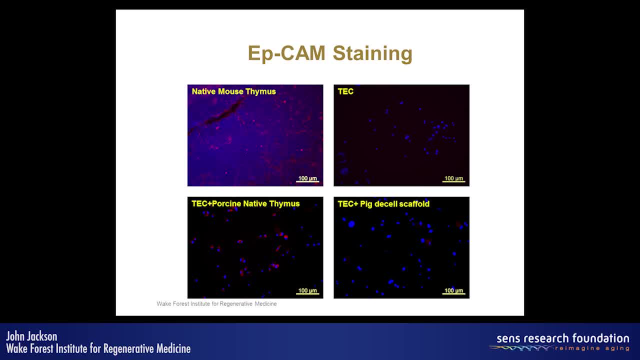 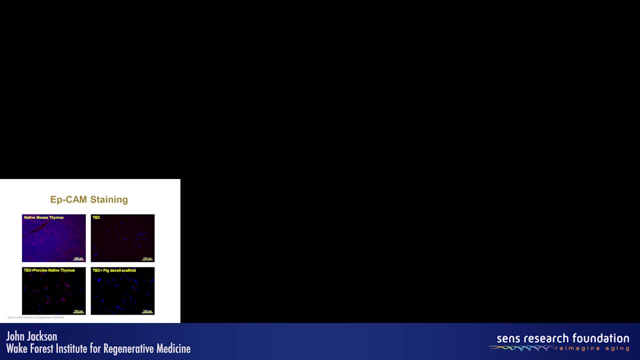 So we then grew epithelial cells and looked at some of the phenotype changes that occur during culture. If you take thymic epithelial cells, place them in culture, they lose their expression of epcam. as you can see here, This is a one-week culture of thymic epithelial cells. 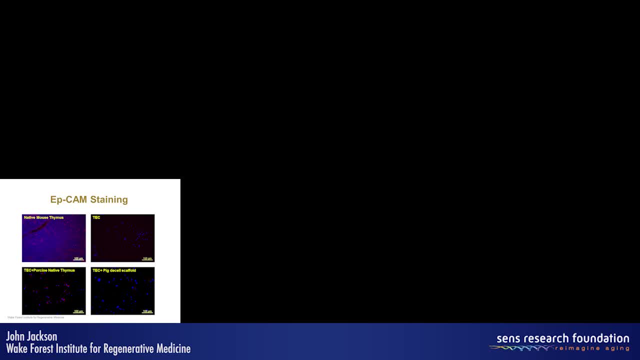 And they don't express epcam. But if you look at whole mouse thymus you can see that there's abundance of thymic epithelial cells expressing epcam. After one week of treatment with the powder from the porcine native thymus we get very nice up-regulation. 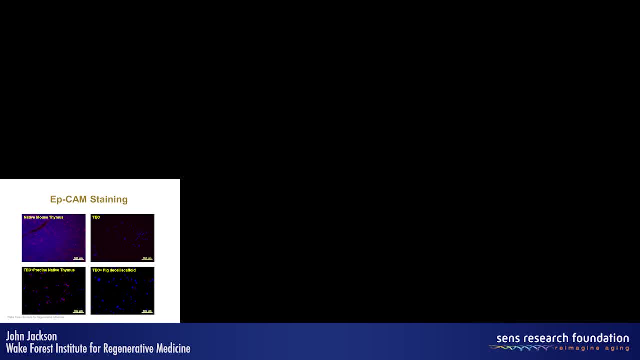 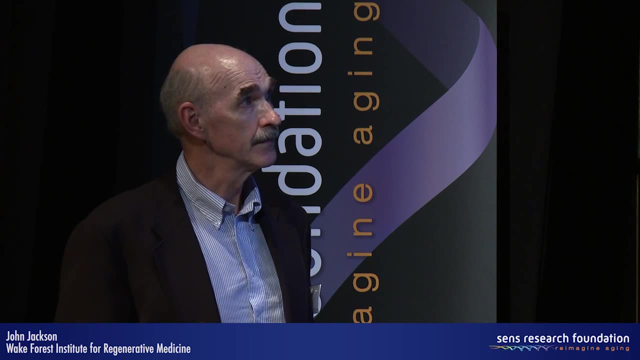 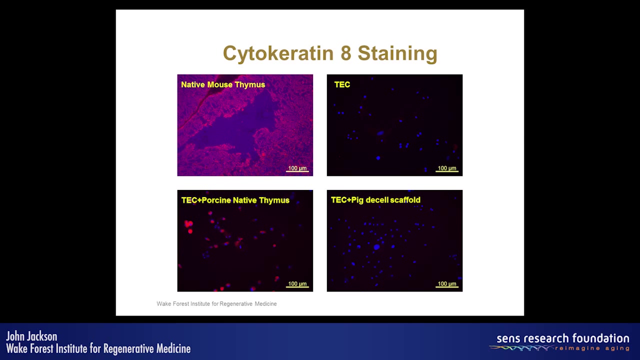 of EPCAM in these cells. If we use the pig decellularized scaffold we see a little bit, but it's not as pronounced as using the whole tissue. cryo-milled powder, Cytokeratin 8, is one of the cytokeratins that is expressed in the 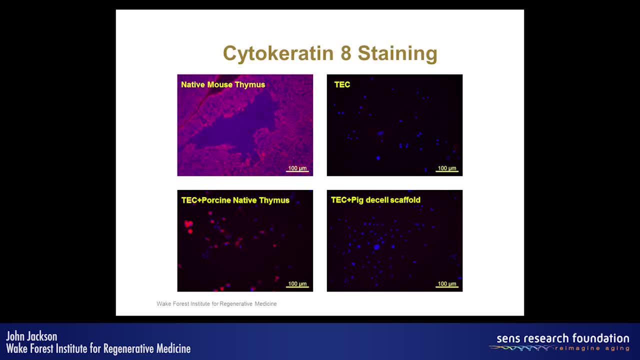 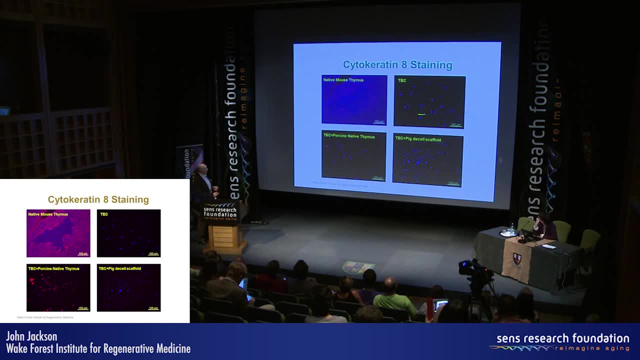 cortical region of the thymus. You can see that very nicely expressed here. This is the medullary region with very little staining of cytokeratin 8.. If you look at thymic epithelial cells, they don't express cytokeratin 8 when you place them in culture. 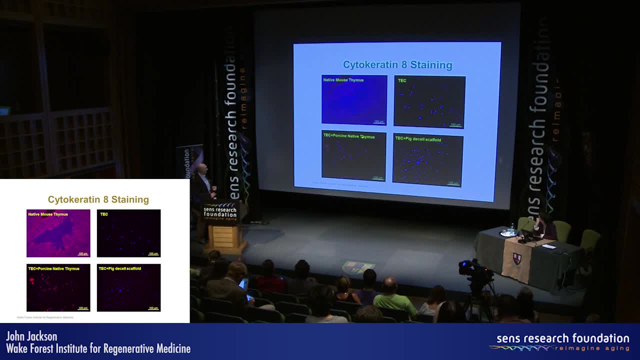 However, after exposure to the native thymus cryo-milled material, you get very nice up-regulation of cytokeratin 8 within these cells. You see a little bit with the decell scaffold. What we're seeing here is probably some of the 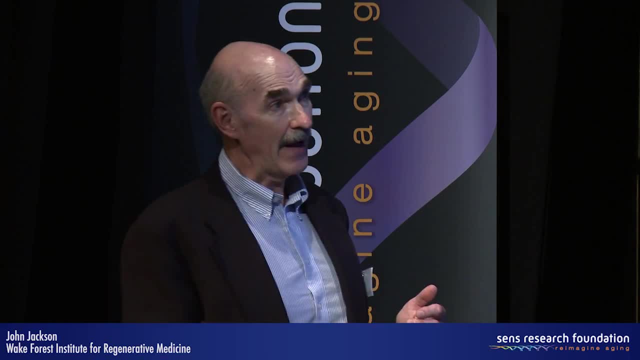 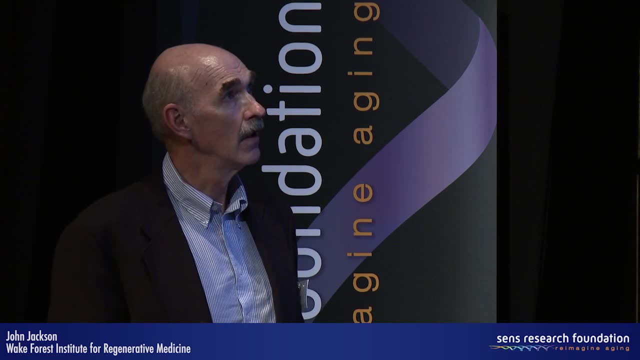 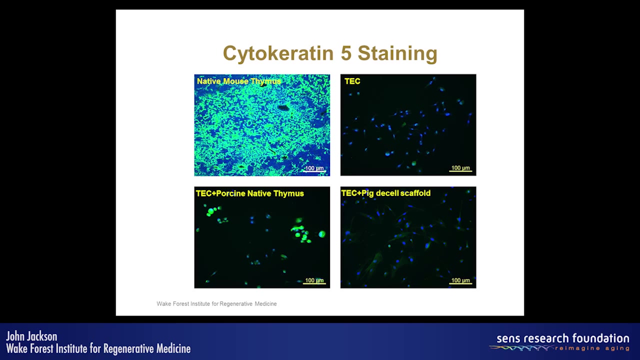 elimination of some of the factors during the decellularization process. Now, if we look at cytokeratin 5, which is expressed in the medullary epithelial cells- the cortical regions are up here- Less expression, more expression in the medullary region. You do see. 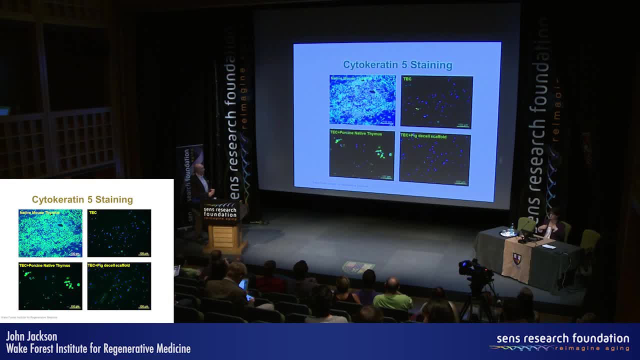 C expression in thymic epithelial cells that have been cultured for a week. But if you add this powder from the native thymus you get much more up-regulation of expression of this particular cytokeratin and you also see some with the pig decell scaffold. 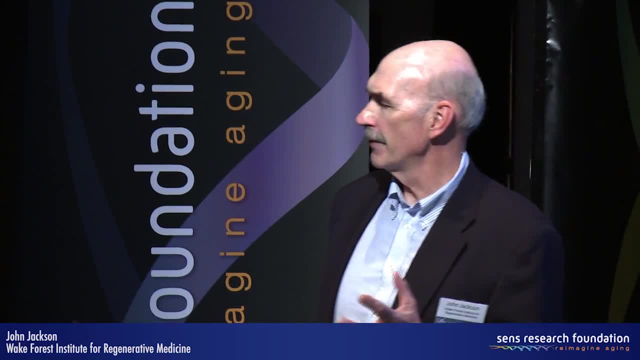 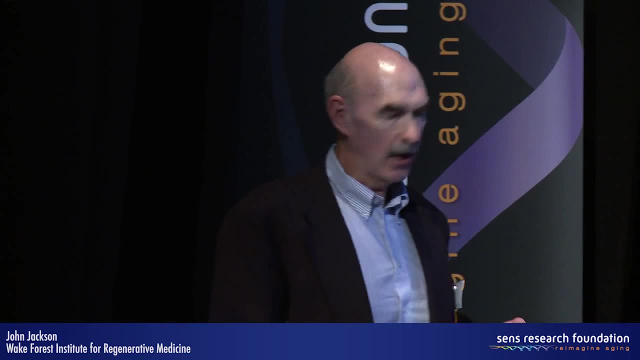 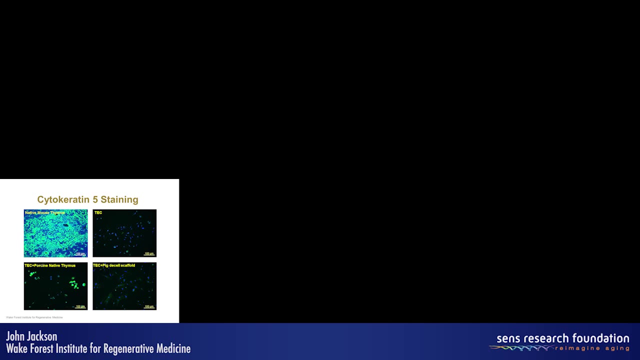 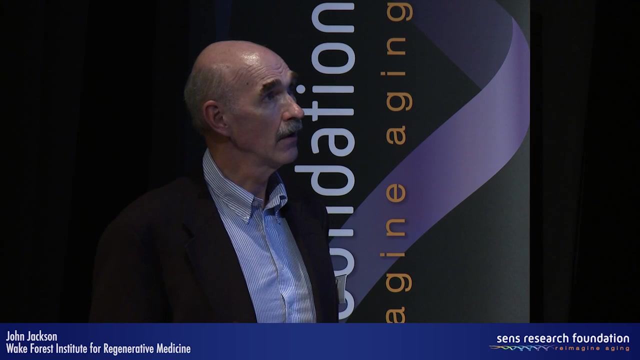 So what we're seeing is this material has the ability to up-regulate the proliferation of the thymic epithelial cells. It also induces and maintains the appropriate expression of these thymic epithelial markers, EPCAM, and the cytokeratins 8 and 5.. 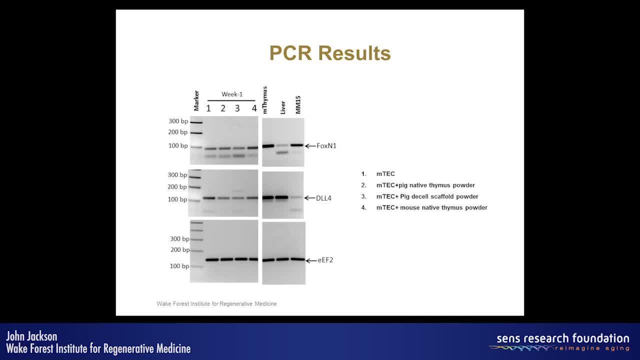 We also looked at the potential up-regulation of some of the important transcriptional factors, in this case FOXN1.. We can see this is native thymus. It decreases if you just place epithelial cells in culture And then in the presence. we can see. 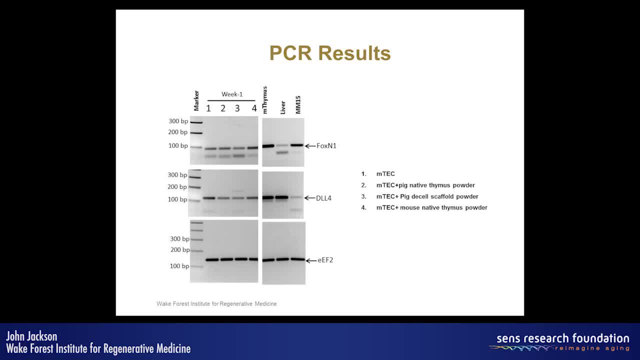 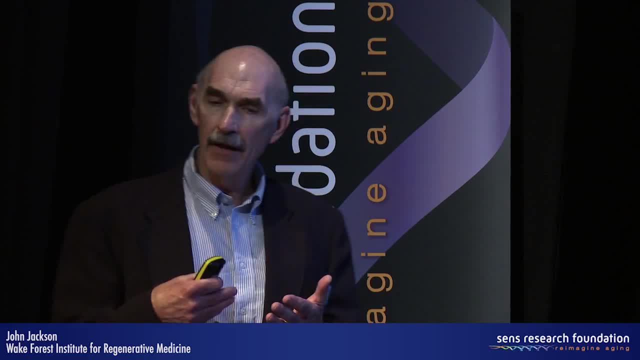 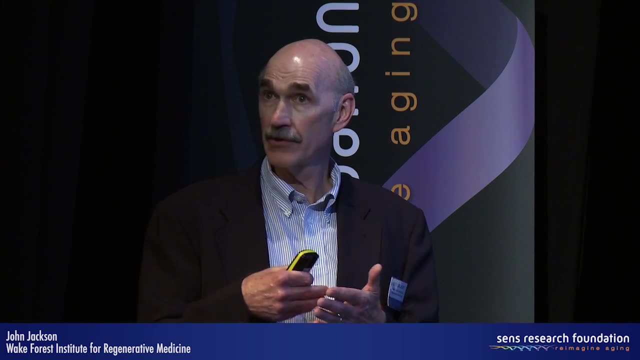 a small increase with the mouse native thymus powder. We expect to see a much greater increase once these epithelial cells have direct contact with bone marrow progenitors or thymus progenitor cells. There is a two-way communication between the epithelial cells and the mouse native thymus. 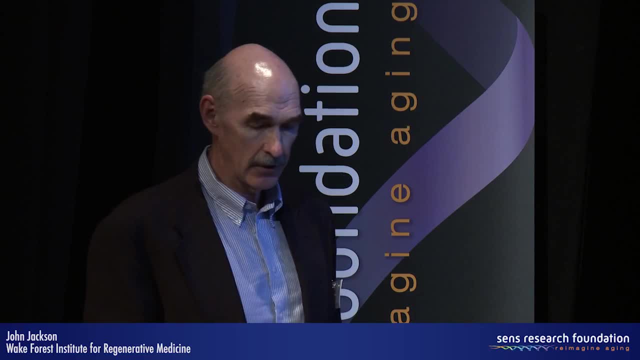 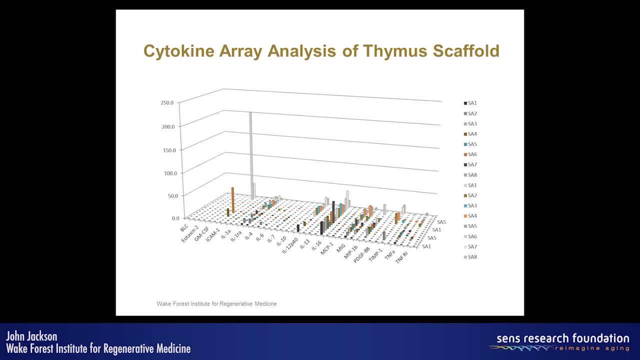 Here we can see both of these response. by accenting 엄마te defender, You can see the bactriaظ Aquio. you can see whatever was contained in the epithelial cell. It is some macrophage that I have also identified. 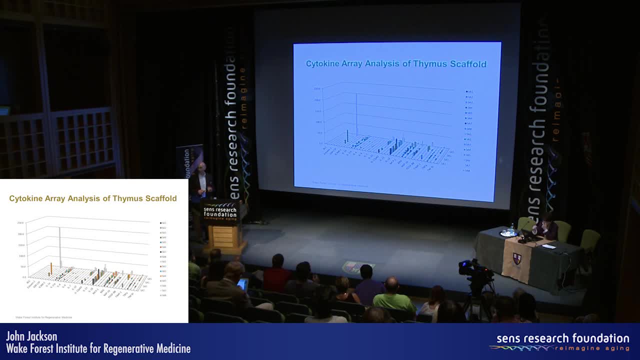 These are different colors, but one of the reasons isn't it that it's a relatively collective association ofbye or bloque che Podaction. We can see that 요, We can find some IL-1 present there, a little bit of GM-CSF. 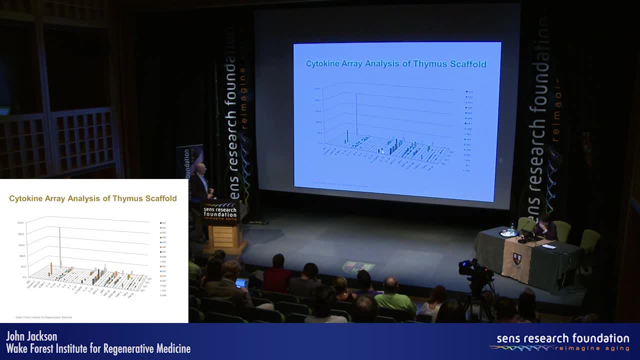 In some samples it's much higher than others. We see IL-12, as well as some chemokines, And these chemokines are very unique in terms of being more specific for T-cells and not macrophages monocytes. 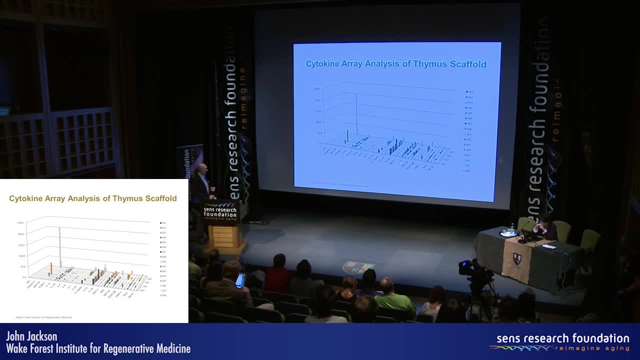 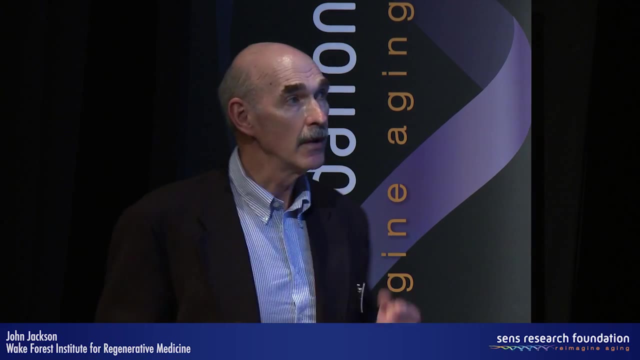 So IL-16, this is a monocyte Inducible interferon, gamma chemokine, as well as MIP1 beta. So all of these are involved in bringing in T-cell populations, So that may be extremely important in terms of recelularization of this scaffold. 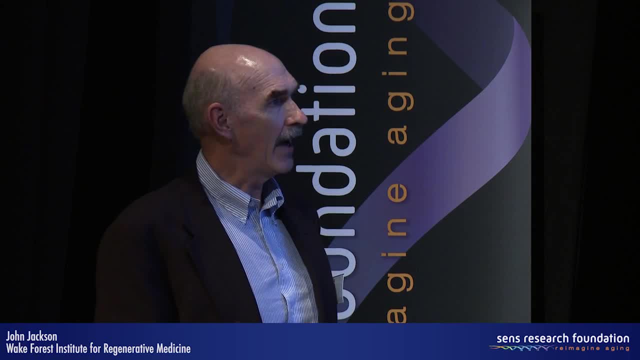 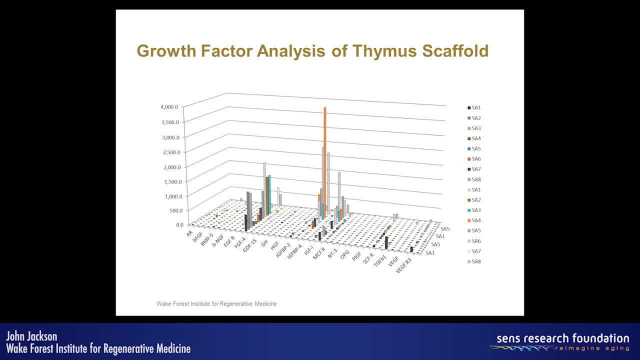 If you look at the growth factor analysis, we have FGF, which is important in terms of looking at epithelial maintenance and growth. We have insulin-like growth factor, as well as some insulin-like growth factor binding proteins that are present in these scaffolds. 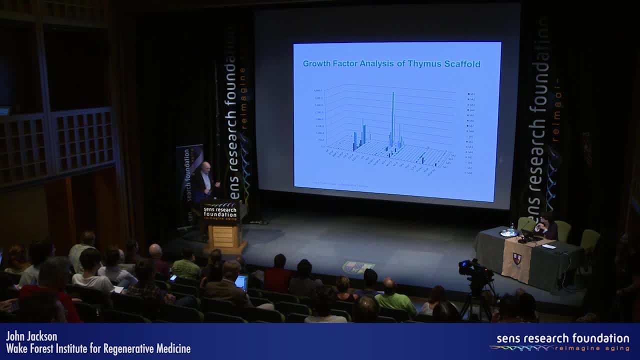 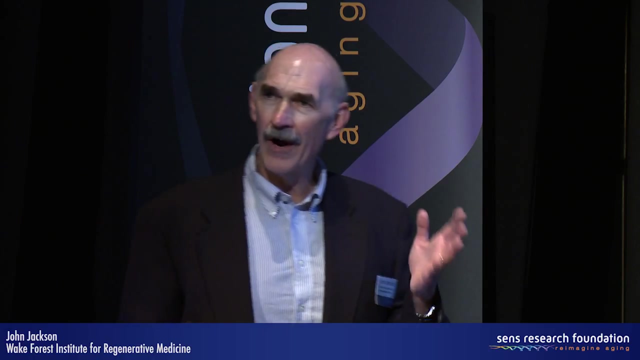 I was a little disappointed in the data. I was expecting to particularly see maybe some IL-7 and some IL-4, other important cytokines which we didn't see, which may be eliminated again during the production of the scaffolds or actually how we acid extrude. 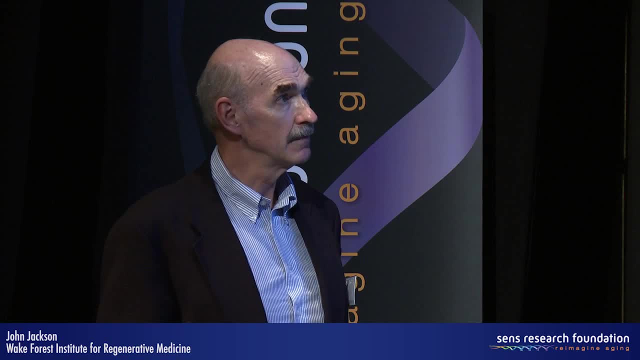 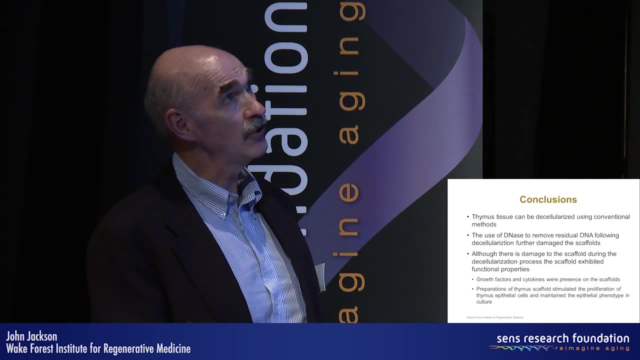 We extracted these to get the cytokine arrays. So actually, in conclusion, we can take thymus tissue. It can be decellularized using standard detergent methods. The use of DNAs to remove the residual DNA further damages the scaffold. So we're actually looking at this very closely.